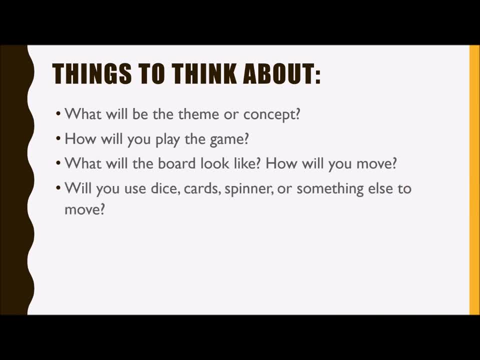 And how will you move? Will you use dice, cards, spinner or something else to move? What will you use as game pieces And how do you win and finish the game? The first thing I want you to decide is: what is the theme or concept of your game. 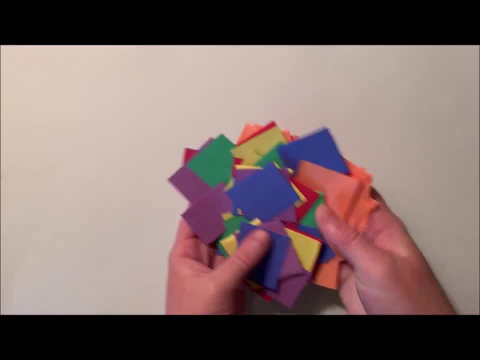 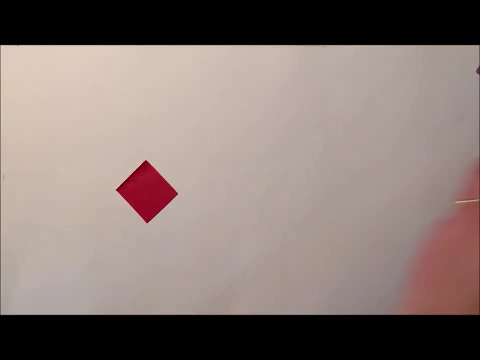 For me, naturally, as an art teacher, I'm making an art game based on colors, So I'm using these squares, a glue stick, sharpie, scissors, a few other things. Next, you need to decide what will look similar to Candyland with all of my colors. 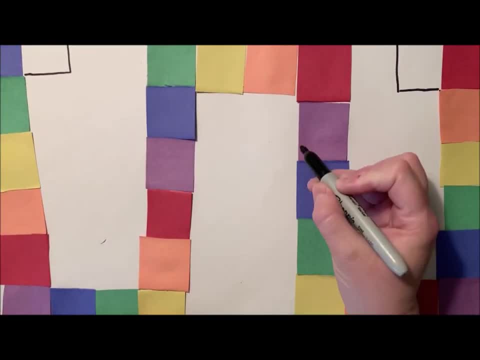 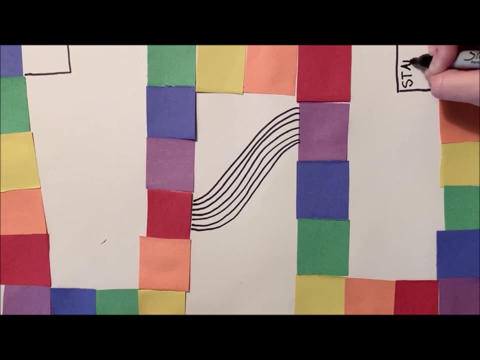 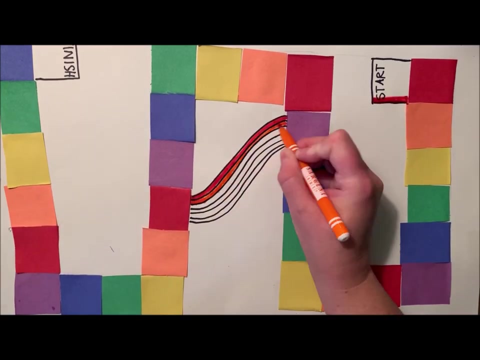 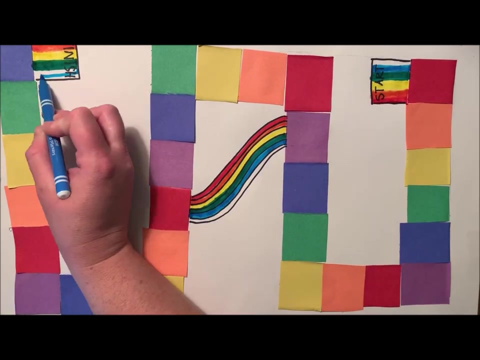 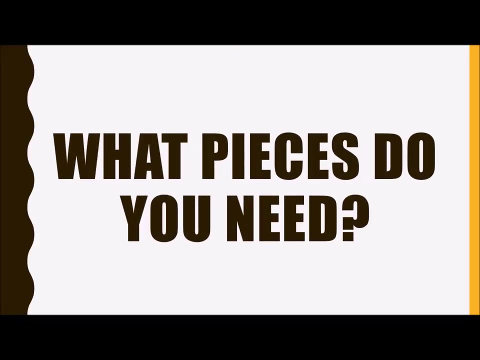 Now that I've designed my path, I'm going to add a start and finish, as well as a rainbow shortcut. I'm just going to test my numbers. Next, I'm going to add a title. My game needs a name. Next, we may need to decide: what pieces do we need? 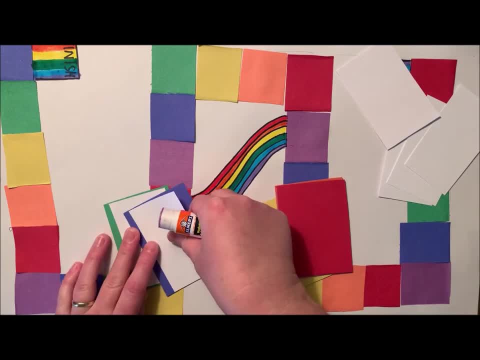 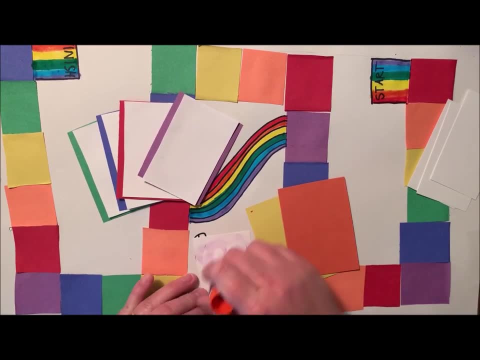 I decided to use cards for every color that you land on. For example, if you land on a green, you'll pick up a green card. Right now I'm putting together the blanks for the cards, along with the colors. 2. Drawing a picture. 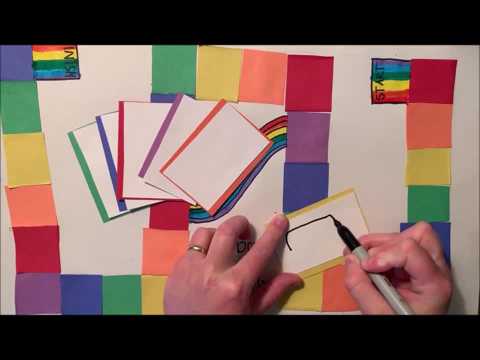 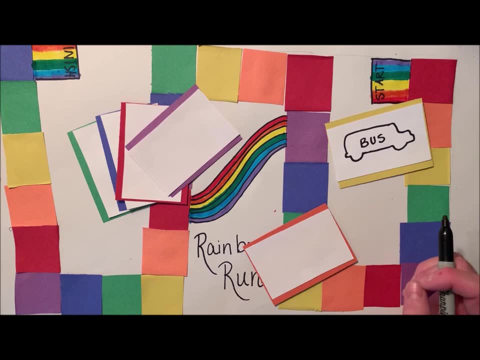 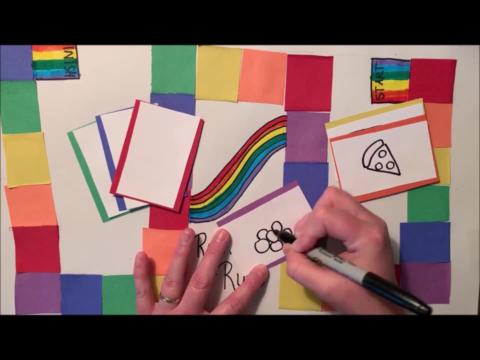 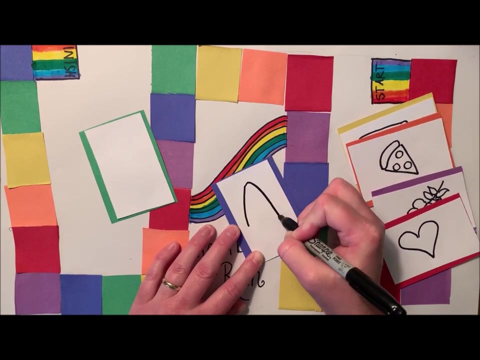 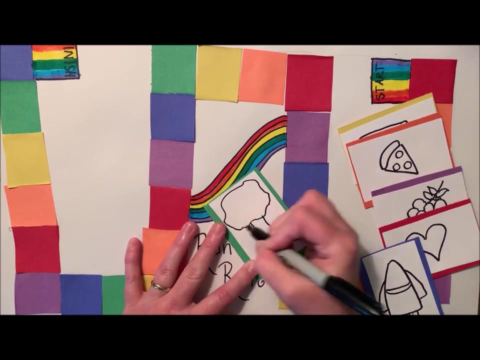 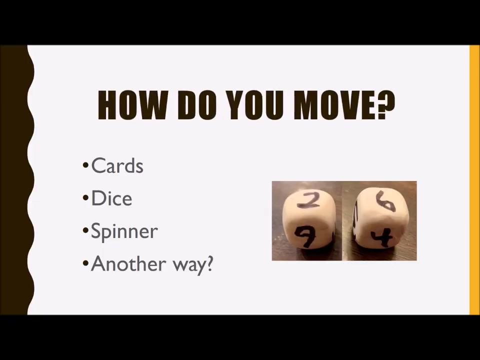 Next, I'm drawing pictures for my rain. submit my game. You'll see what they're for in a minute. Now that my cards are complete, I'm ready to play the game. Just a couple more things. How are you going to move on the game? I decided to use dice for mine, So I put the cards down. 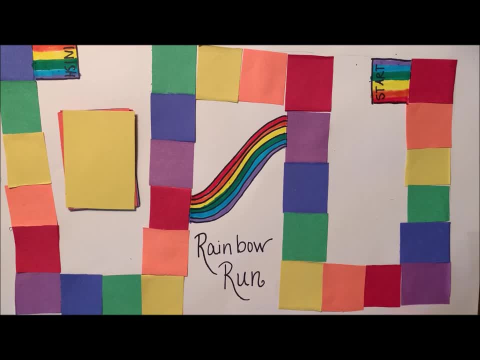 on my game board, I grab my dice. This is used to roll and determine how many spaces you move, And I also have my players. Now, since it's an art game, I decided to use some art supplies for my game. I'm going to start out by using the